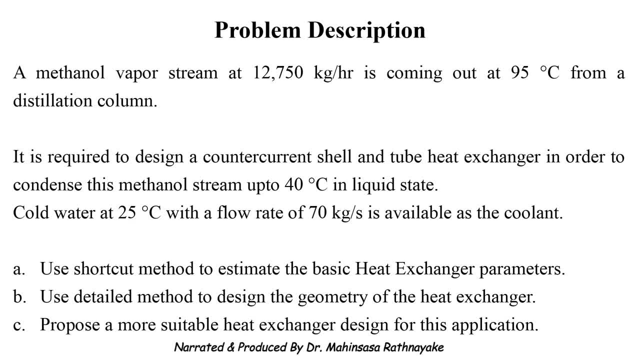 A methanol vapor stream at 12,750 kilograms per hour is coming out at 95 degrees Celsius from a distillation column, It is required to design a counter current shell and tube heat exchanger in order to cool down this methanol stream up to 40 degrees Celsius. 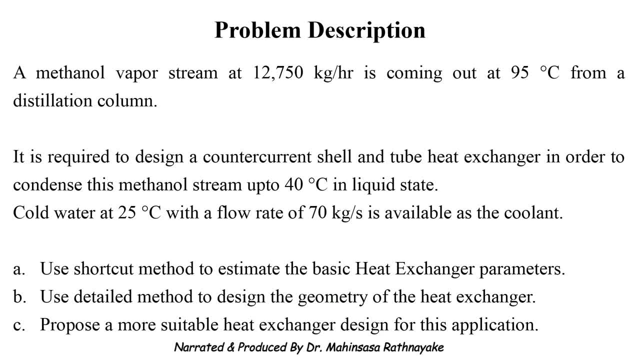 In liquid state. Cold water at 25 degrees Celsius with a flow rate of 70 kilograms per second is available as the coolant. First we need to use the shortcut method to estimate the basic heat exchanger parameters. Then we need to extend our design using the detailed method. 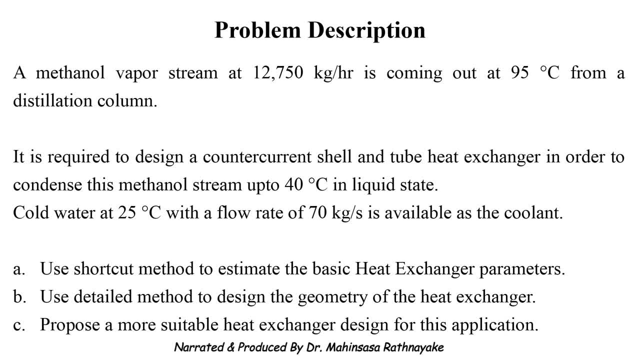 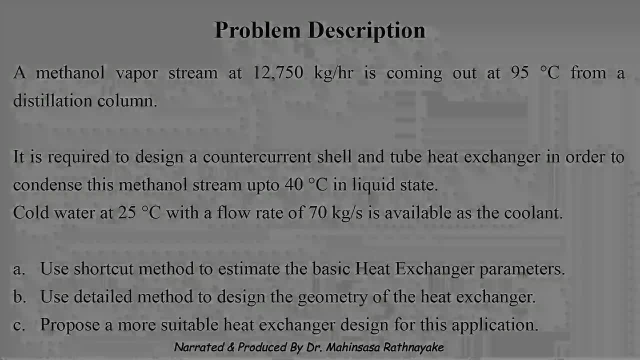 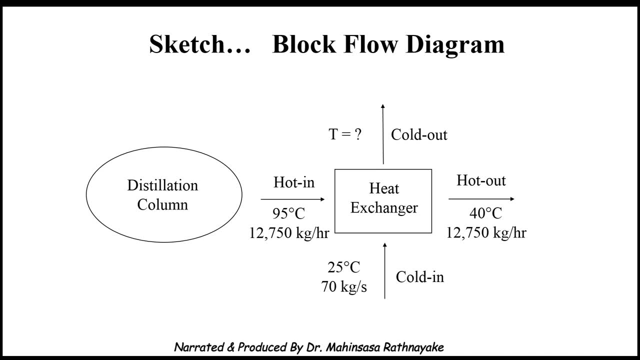 to design the geometry of the heat exchanger. Based on the results, we need to propose a more suitable heat exchanger design for this application. It is a good habit to sketch the block flow diagram before starting to solve a design problem According to the problem statement. 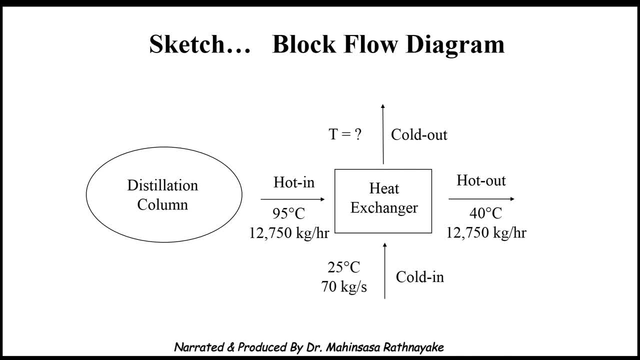 hot methanol stream enters the heat exchanger at 95 degrees Celsius with a flow rate of 12,750 kilograms per hour. The methanol stream is in vapor state and it must be condensed and cooled down up to 40 degrees Celsius. The cooling water enters at 25 degrees Celsius with a flow rate of 70 kilograms per second. 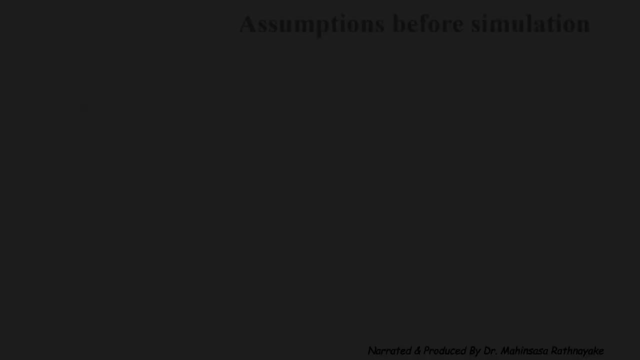 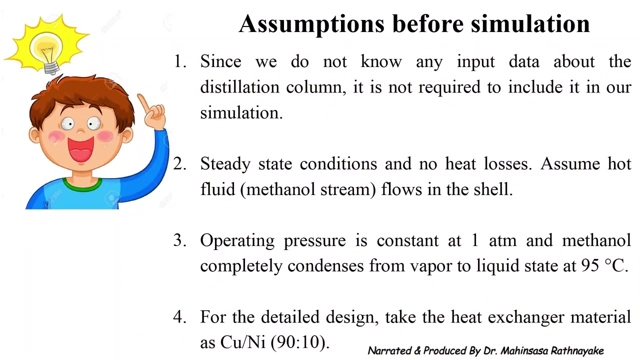 And the cold water outlet temperature is unknown. As engineers, we must make valid assumptions to solve the problems easily. Keep in mind that if you want to be a good engineer, you must develop good imagination skills. We can have these assumptions for this problem to make our calculations easy. 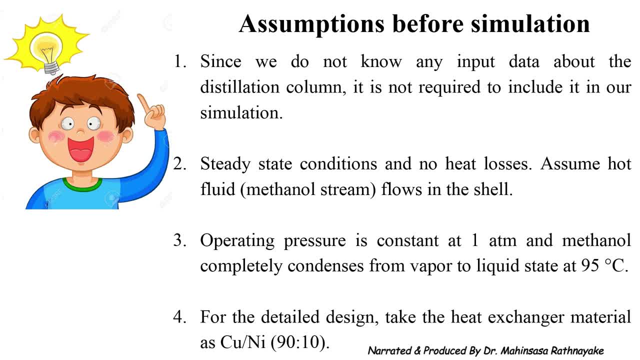 Since we do not know any input data about the distillation column, it is not required to include it in our simulation. We can assume steady state conditions and no heat losses. As well, we can assume hot fluid flows in the shell. Let's take operating pressure is constant at 1 atm. 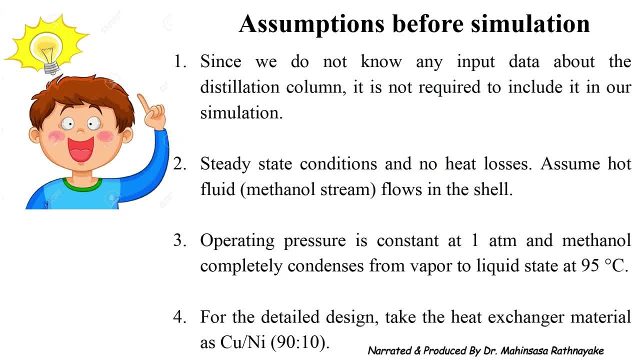 and methanol completely changes from vapor to liquid state. For the detailed design, let's take the heat exchanger material as copper alloy with 10% nickel. Before starting the simulation with Aspen Plus, let's have a look at the manual solution of this problem. 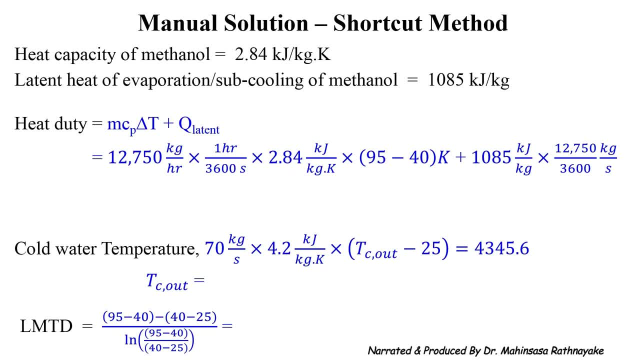 First, using the shortcut method, we can find out the heat duty for this heat exchanger. For the heat duty we need to account the latent heat of sub cooling of methanol, Because initially methanol is in vapor state. So we can calculate. the total heat duty is equal to: 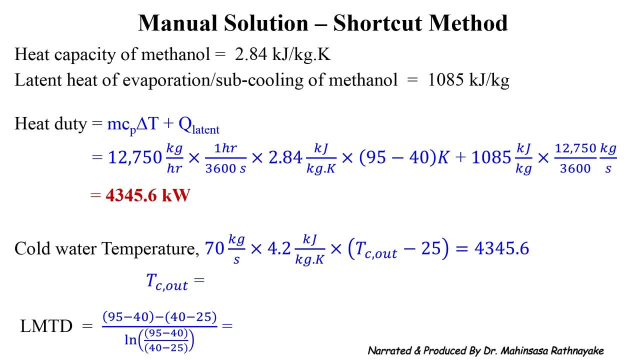 4,345.6 kilowatt. Using the calculated heat duty, we can estimate the cold water outlet temperature is almost equal to 40 degrees Celsius As well. we can calculate the logarithmic mean temperature difference is equal to 30.8 degrees Celsius. 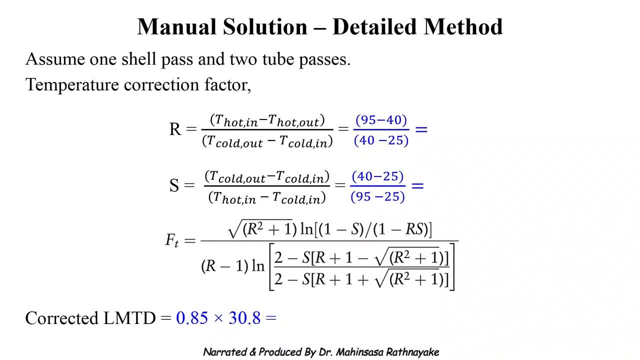 In the manual detailed design method, we need to first find out the temperature correction factor for LMTD. In order to find out the temperature correction factor, first, we need to estimate the two correlations R and S. Using the given equations, we can calculate these correlations as: 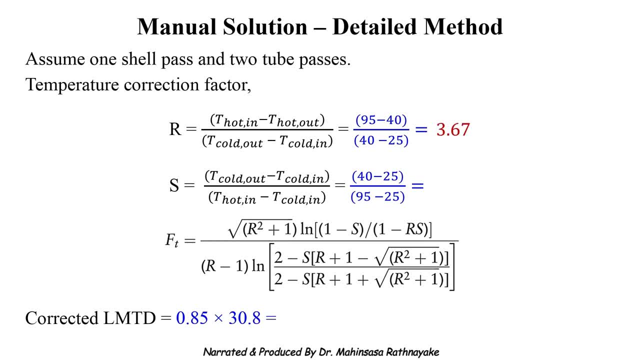 R is equal to 3.67 and S is equal to 0.21.. Using these values of correlations, we can find out: the temperature correction factor is equal to 0.85.. Therefore, we can find out: the corrected logarithmic mean temperature difference is equal to 26.18.. 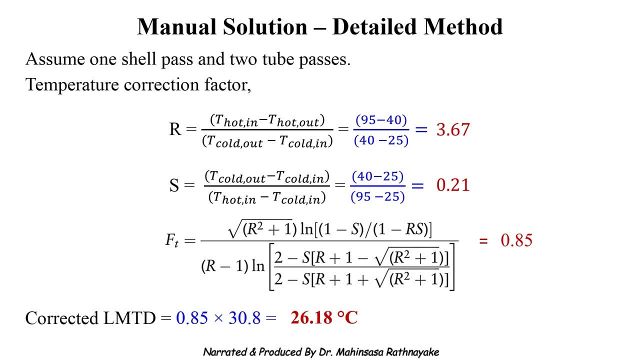 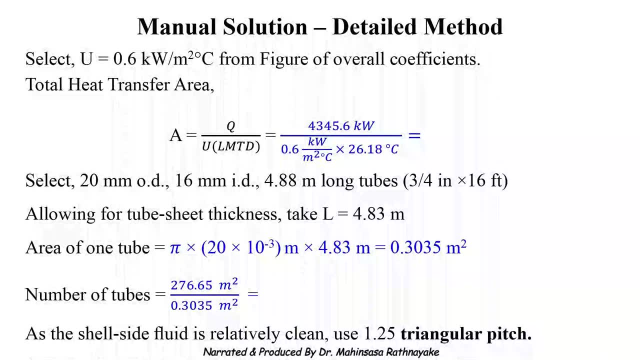 For this detailed heat exchanger design, let's assume one shell pass and two tube passes. In order to estimate total heat transfer area, first we select overall heat transfer coefficient for this heat exchanger as 0.6 kilowatts per square meter per degree Celsius. 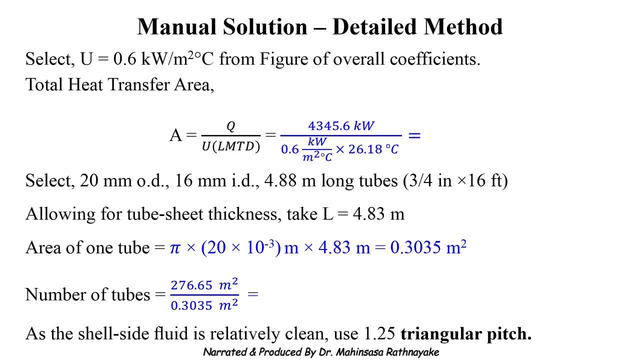 The overall heat transfer coefficients for each process liquids can be found out using the tables and charts. Using the selected overall heat transfer coefficient and the corrected LMTD value, we can estimate the total heat transfer area is equal to 276.65 square meters. 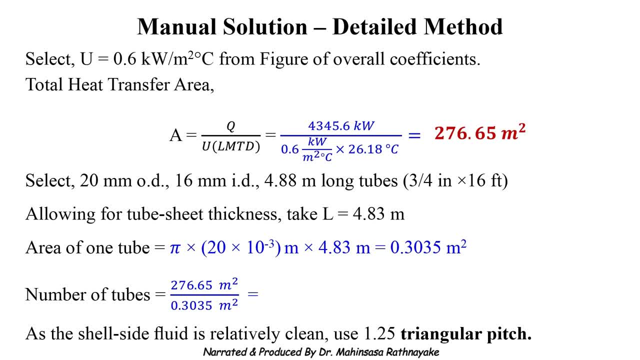 For the tube design, let's select 20 mm outer diameter and 16 mm inner diameter, 4.88 meter long tubes. These tube sizes are coming from standard tube sizes available. This selected tube can be indicated as 3 quarter inch diameter and 16 feet long standard tube. 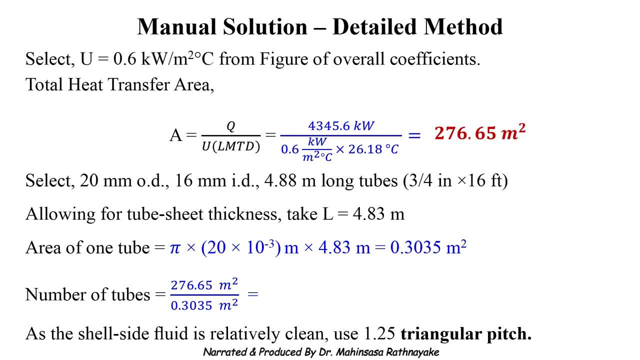 For the tube sheet thickness we can allow 50 mm, so we can take the total length as 4.83 meters Using this selected tube sizing. we can calculate the area of one tube as 0.3035 square meters Using the previously estimated total heat transfer. 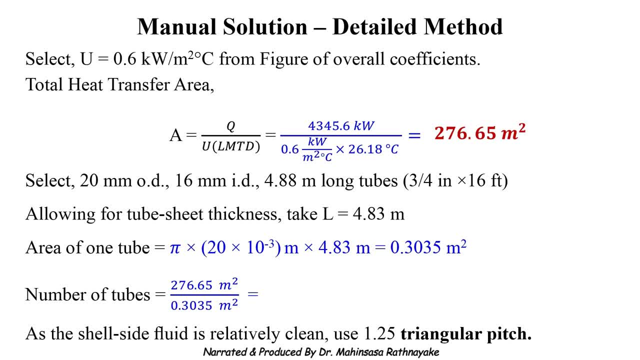 we can estimate the total number of tubes required is equal to 912.. Furthermore, we can decide the shell side fluid is pure methanol and it is relatively clean. We can take 1.25 triangular pitch for the tube arrangement, As we estimated the total number of tubes required. 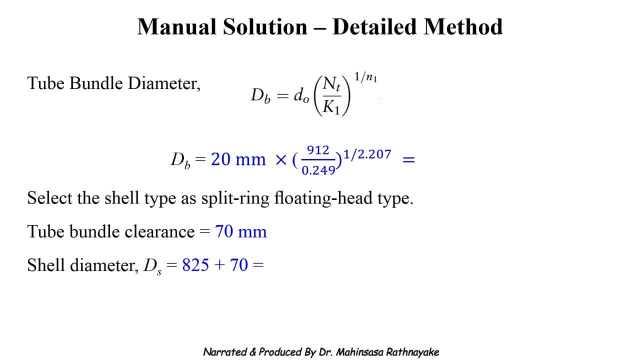 using the equation, we can find out. the tube bundle diameter is approximately equal to 825 mm. We can select the shell type as split ring floating head type. This shell type should be selected based on our application. For the selected shell type, the tube bundle clearance can be found out using the chart. 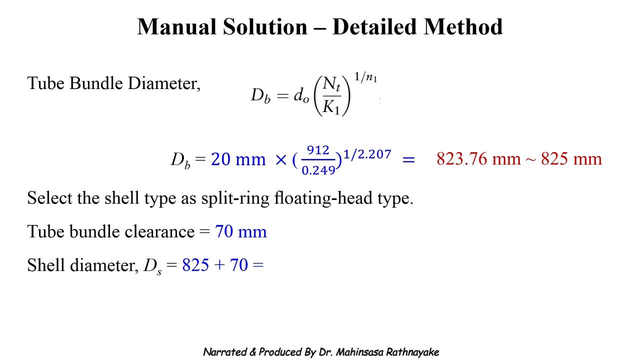 The tube bundle clearance can be taken as 70 mm, So the final shell diameter becomes 895 mm. However, the nearest standard pipe size is 914.4 mm. that is equal to 3 feet. Therefore, we can take the final shell diameter as 914.4 mm. 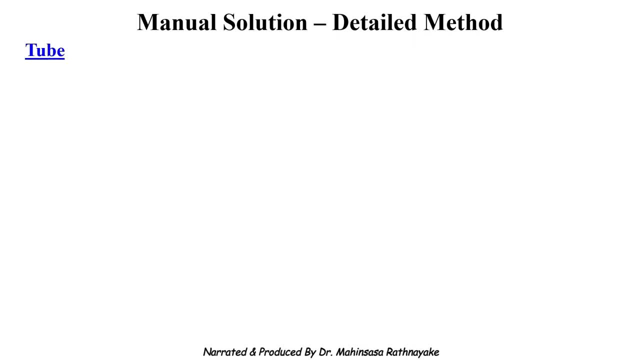 In order to find out the corrected overall heat transfer coefficient based on the geometry of heat exchanger, first we need to find out the tube side coefficient. We can find out: the mean tube side temperature is equal to 32.5 degree Celsius. The tube cross sectional area is equal to 201 mm2.. 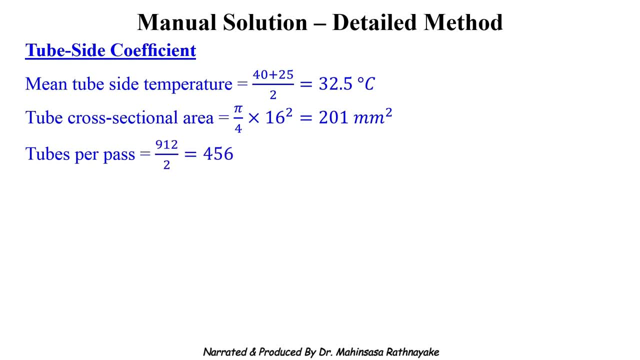 Since we have two tube passes, the number of tubes per pass is equal to 456.. Therefore, the total flow area is 0.0917 square meters. Cold water is flowing through the tubes. Therefore, we can calculate: the cold water mass velocity is equal to 763.36 kg per square meter per second. 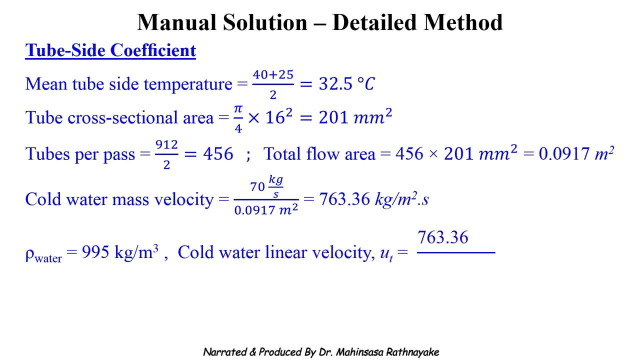 Since the density of water is 995 kg per cubic meter, cold water linear velocity can be calculated as 0.767 meters per second. These calculated parameters can be substituted to the equation to find out the inside fluid film coefficient for the tube side. 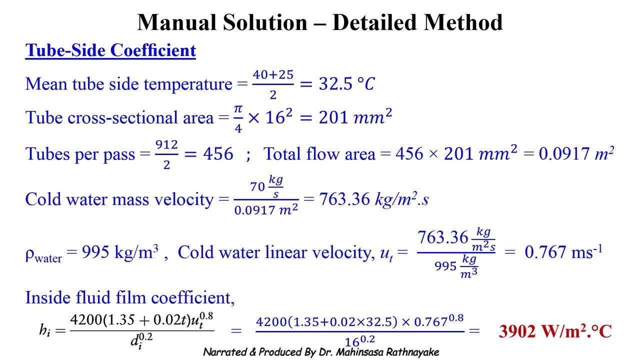 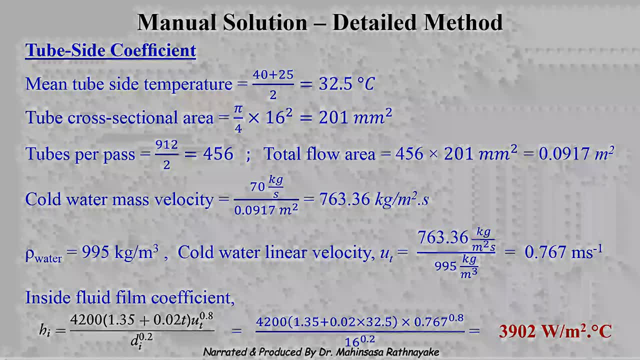 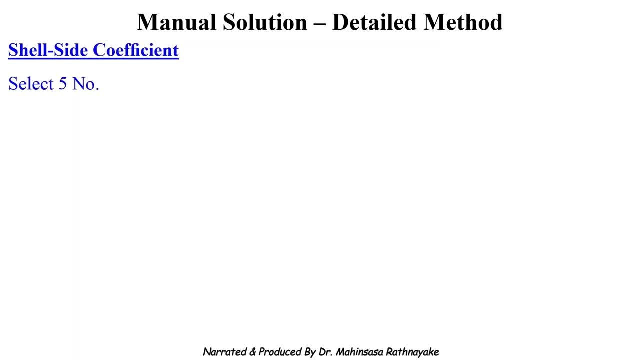 We receive the tube side fluid film coefficient as 3902 Watt per square meter per degree Celsius. Then we should calculate the shell side coefficient. Let's select five numbers of baffles. Generally we select baffle spacing as one fifth of the shell inside diameter. 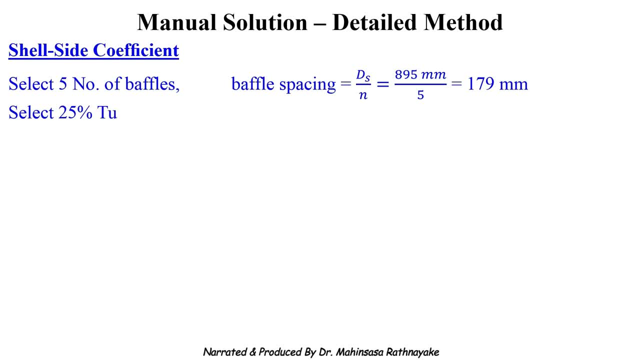 So we can obtain the baffle spacing as 179 mm. Select 25% tube pitch, So the distance between centers of two adjacent tubes becomes 25 mm. Cross flow area for the shell side fluid flow can be calculated as 0.032 square meters. 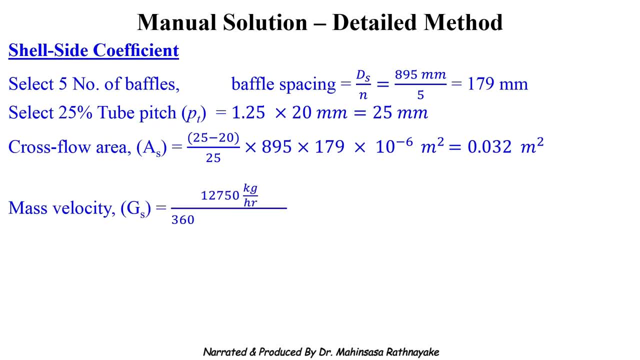 The mass velocity or mass flux can be obtained by dividing shell side mass flow rate by the cross flow area. We receive the answer as 110.68 kg per second. As well, we can find the equivalent diameter required for the calculation of Reynolds number for the shell side using the given equation. 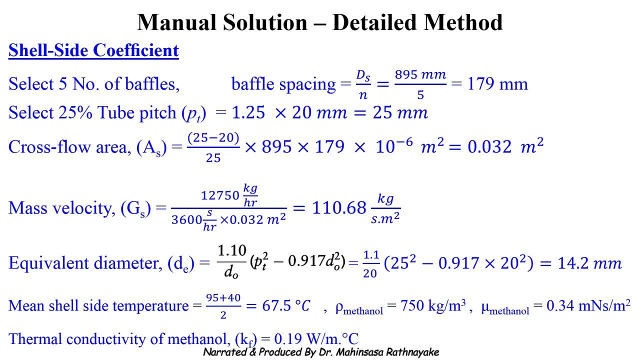 The equivalent diameter becomes 14.2 mm. Average shell side temperature is 67.5 degrees Celsius. Take the density of methanol as 750 kg per cubic meter. Viscosity as 0.34 mN second per square meter. 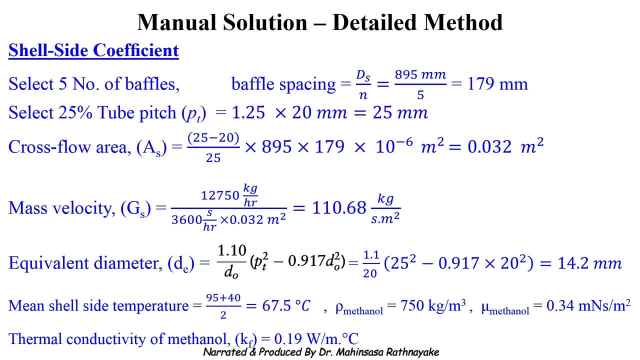 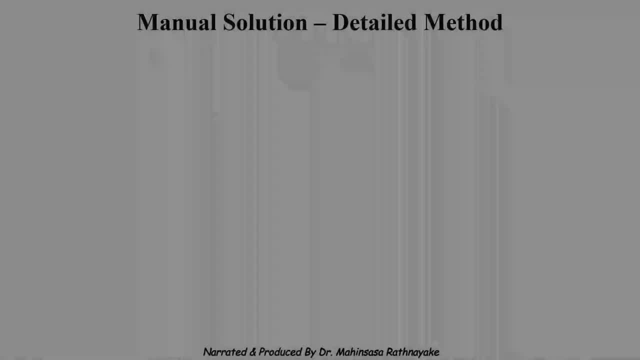 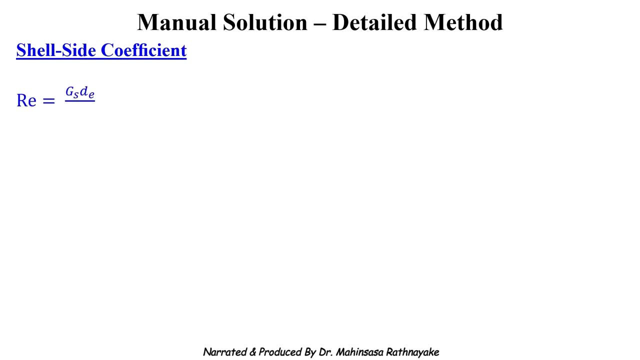 Thermal conductivity of methanol as 0.19 Watt per meter per degree Celsius. Using all these parameters, we can find out the shell side Reynolds number as 4622.5 and Pranal number as 5.1.. Let's neglect the viscosity correction for the shell side coefficient, as methanol is a low viscose liquid. Let's select 25% buffer cut. Therefore, using the graph and the calculated Reynolds number, we can find out: the shell side heat transfer factor is 0.008.. We can calculate the steel side flow rate as 15.29mHg, divided by the heat transfer factor as 15.35.. 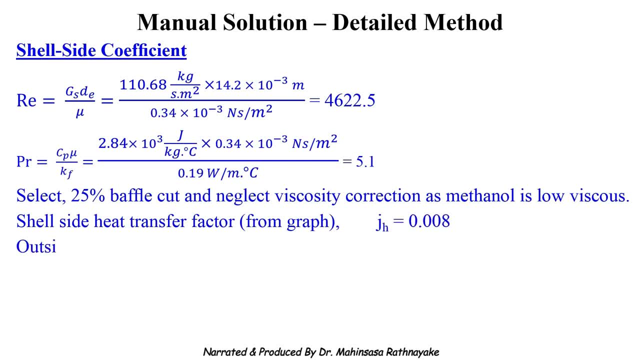 We can go back to the canvass and calculate the flow rate. We can calculate the flow rate by Using the graph again and again. Let's calculate the heat transfer factor as 15.26 mHg per second. Let's go back to the canvass. 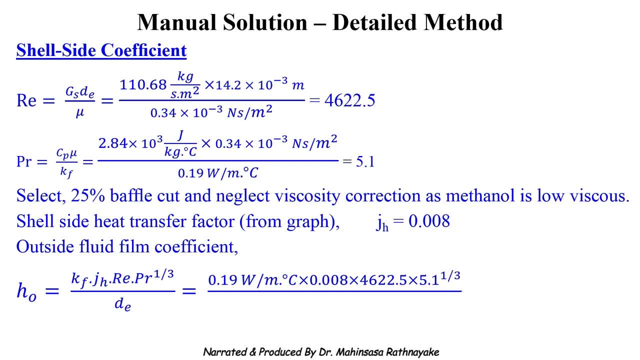 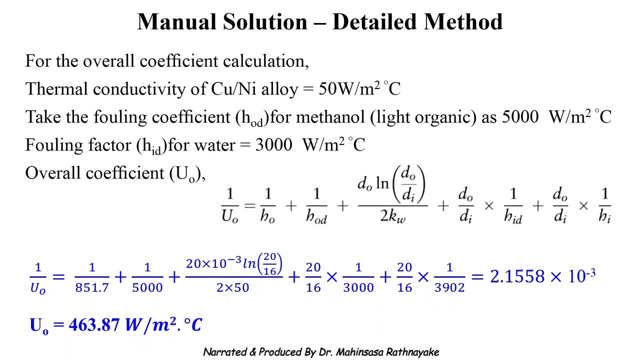 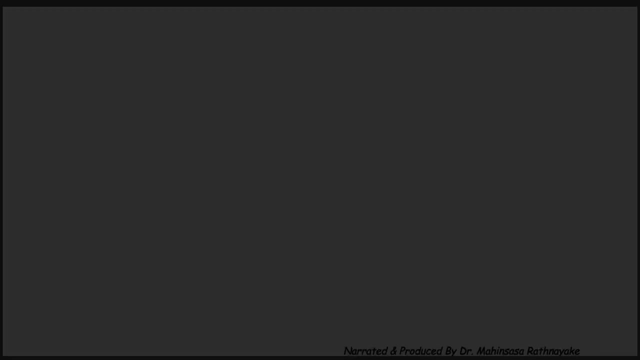 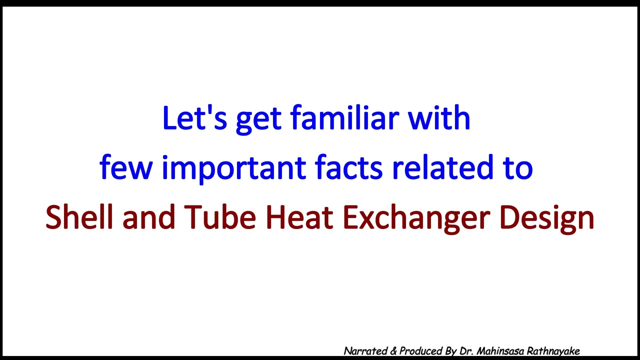 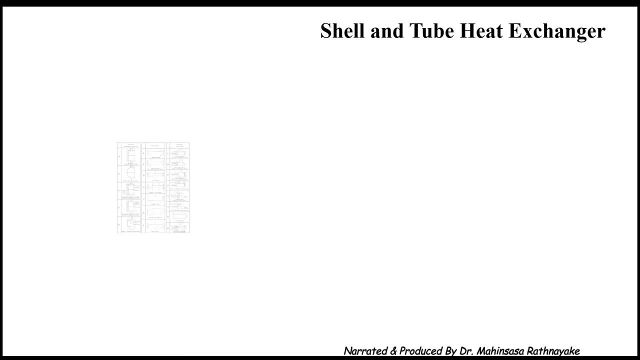 851.7 watt per square meter per degree Celsius. We can plug in all the obtained parameters into the overall coefficient equation and obtain the overall coefficient as 463.87 watt per square meter per degree Celsius. For heat exchanger design generally we use TEMA standard. 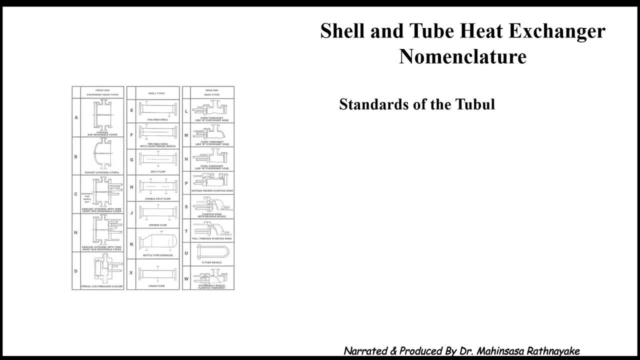 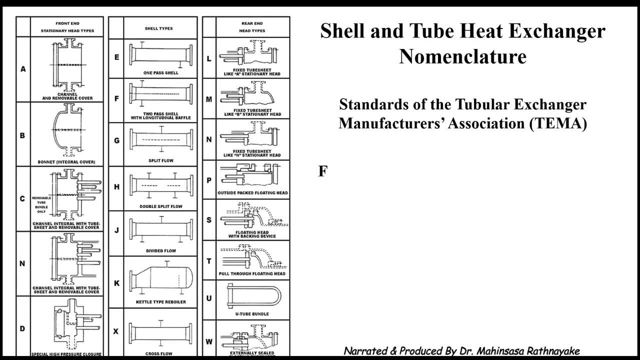 TEMA stands for Tribular Exchanger Manufacturing Association. Let's get familiar with few important facts about TEMA standards in order to improve our heat exchanger design abilities. Let's take a look at some facts about checked current in heat exchanger in a microwave until. 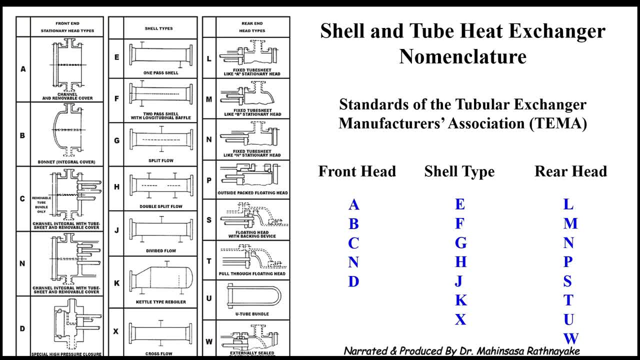 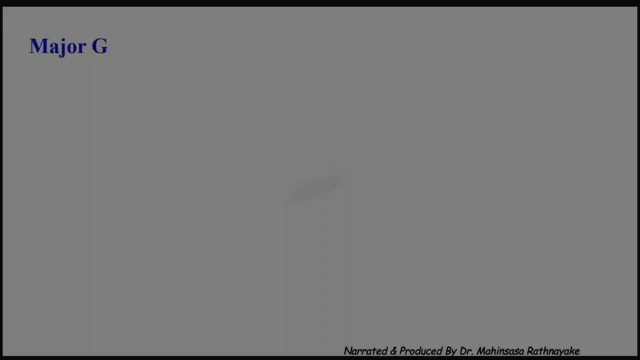 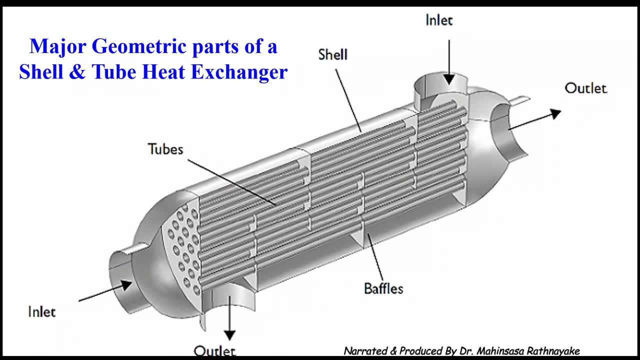 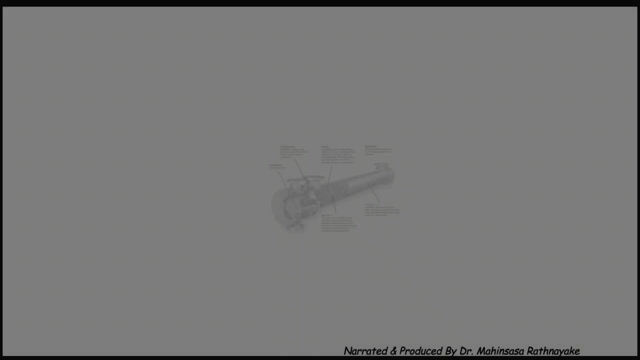 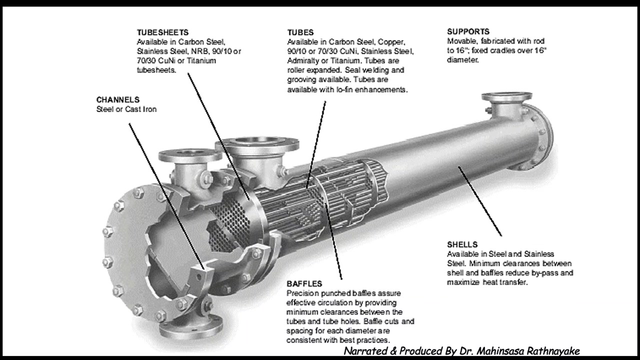 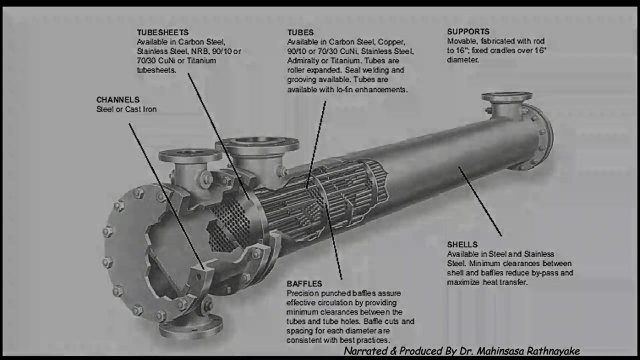 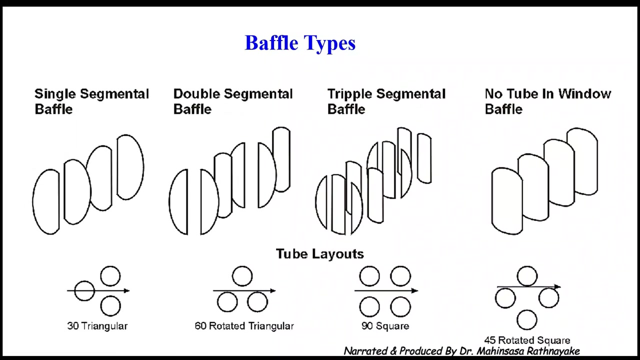 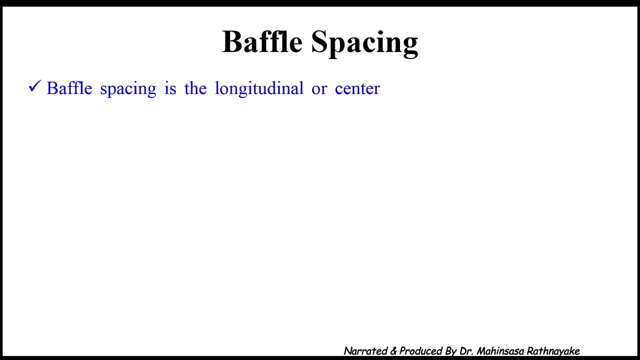 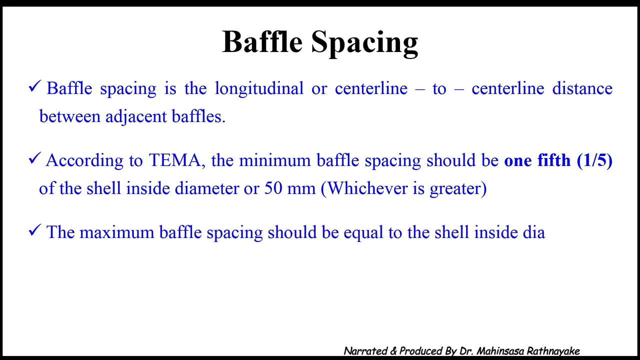 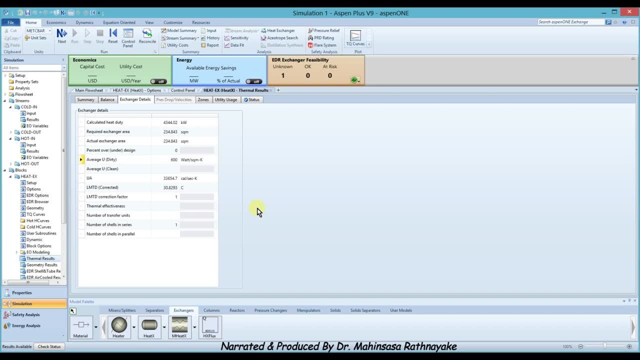 Note that in order to determine the most suitable geometry for the heat exchanger, in actual heat exchanger design, it is required to check the geometric design provided by the mechanical engineers. This checking is referred as heat exchanger rating. If we use manual calculations, we may have to spend a lot of time on multiple calculations. 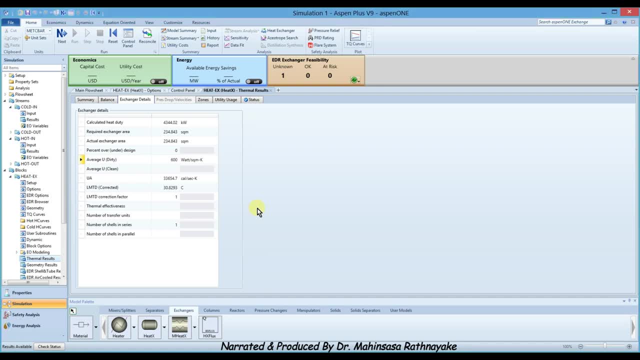 with many new geometries of the heat exchangers in order to end up with the most suitable design. However, this task is very easy when we use a simulation program like Aspen Plus. Aspen provides a separate program called Aspen Exchanger Design and Rating, abbreviated as: 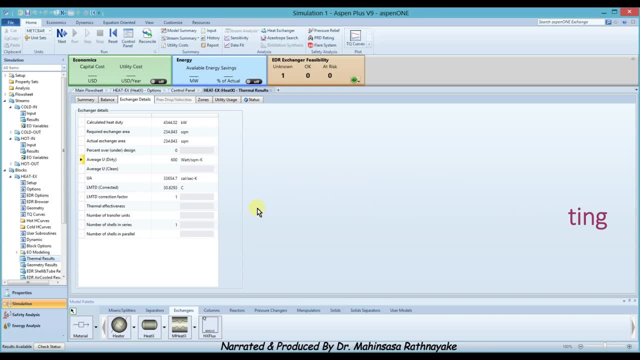 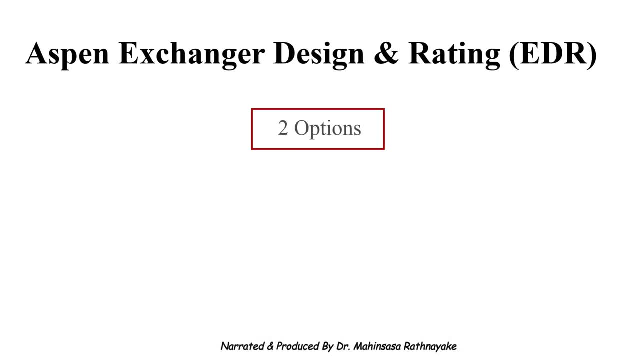 EDR in order to support this requirement. There are two methods to simulate heat exchanger geometry. First option is generating the design in EDR program and use the saved design geometry. Next, we need to find the heat exchanger geometry. Use the saved design file directly into Aspen Plus heat text block. 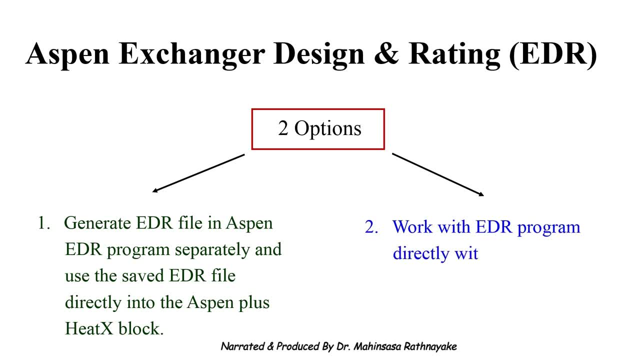 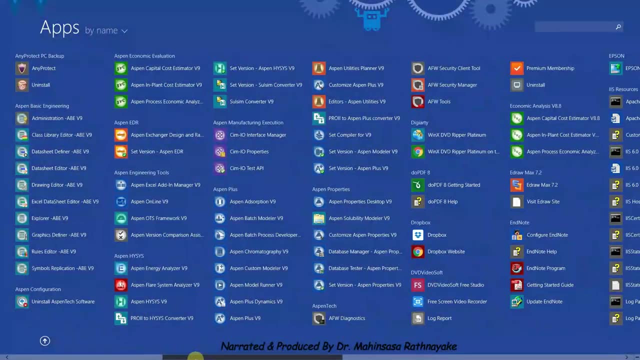 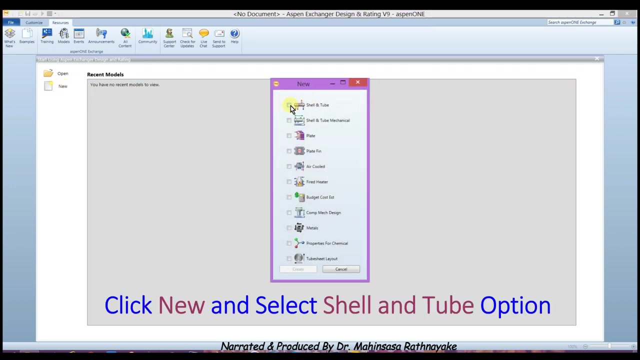 The second option is working with EDR program directly within Aspen Plus simulation. In this example we will see the first option, So let's open Aspen Plus EDR program. It is available in the list of installed applications in your computer, So open Aspen Exchanger Design and Rating program. 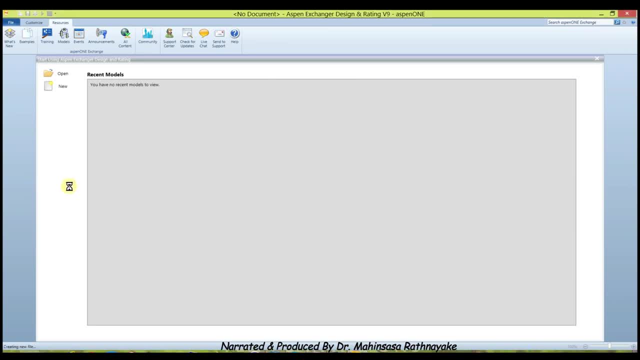 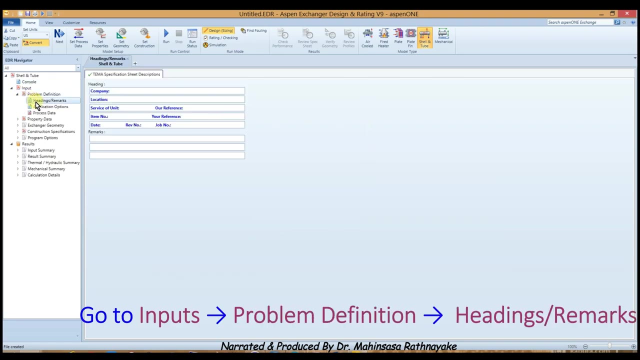 Click New and select Shell and Tube. Then click Create In the EDR Navigator tab. expand the Input Program Definition tab. Click on Headings Remarks tab. For our design we can enter the documentation details like company name, address and date. 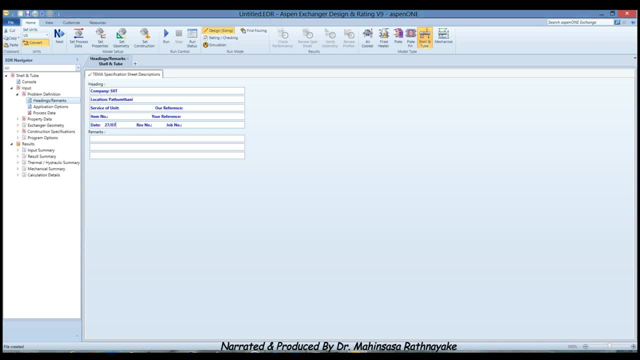 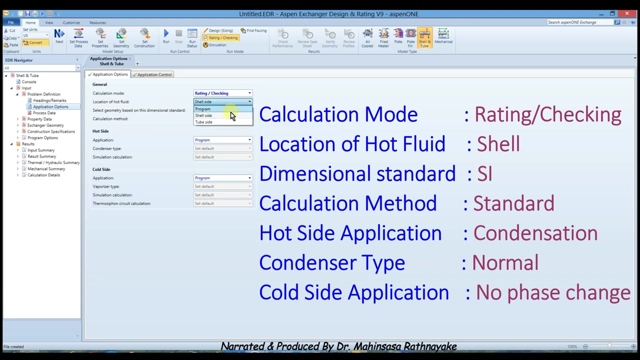 Then go to Application Options tab, Since we need to check our manually created design in this simulation. change the Calculation mode as Rating Checking option. Assign the location of hot fluid into Shell. Change the job name, Change the geometry into SI units, Then change the calculation method as Standard method. 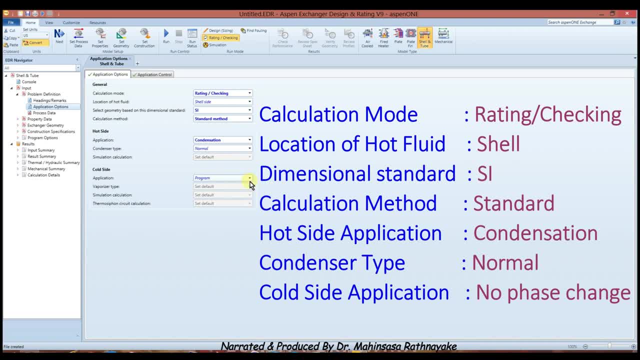 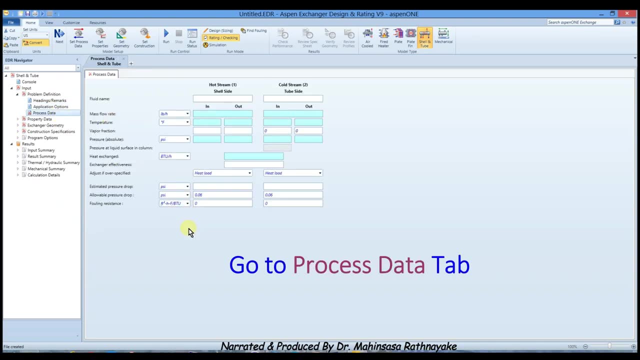 Our application is Condensation of Methanol. Therefore change Hot side application as Condensation and Condenser type as Normal. Change the cold side application as Liquid. no phase change. After that go to Process Data tab Name: Shell side fluid as Process Liquid and Tube side fluid as Cooling Water. 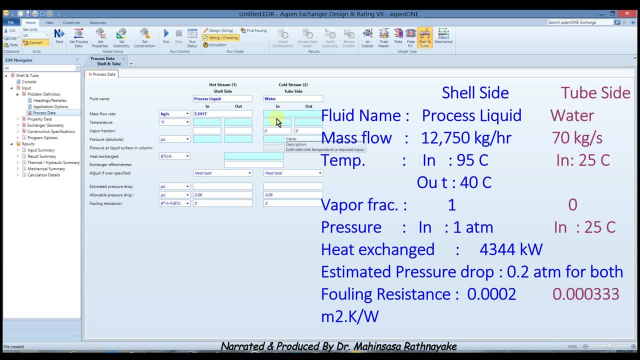 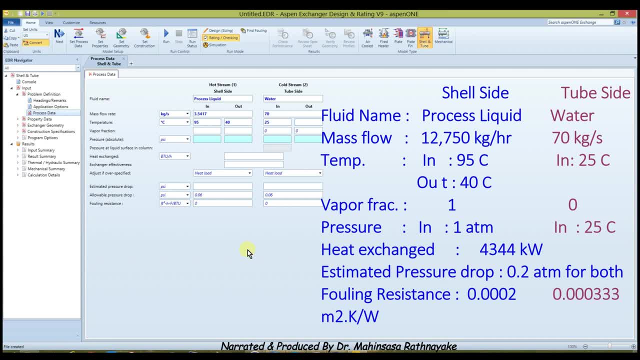 Enter in and out temperatures accordingly. Enter the hot stream inlet vapour fraction as 1 and other vapour fractions as 0.. Enter the inlet pressures as 180M and for the moment, keep the outlet pressure as default. Enter the heat exchange as 4344 kW. 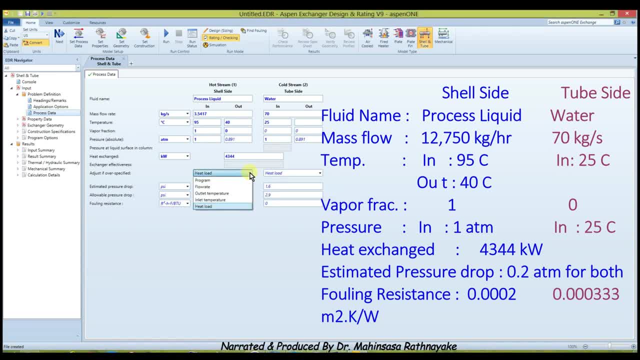 Set outlet temperature to be adjusted if over specified. Enter estimated pressure drop as 0.2 atm for both sides. Enter the falling resistances of methanol as 0.0002 m2 KW and water as 0.000333 m2 KW. 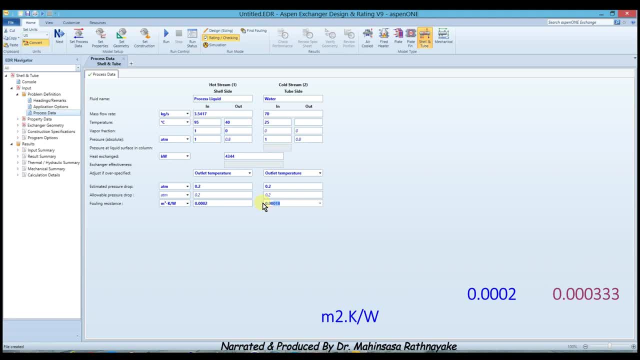 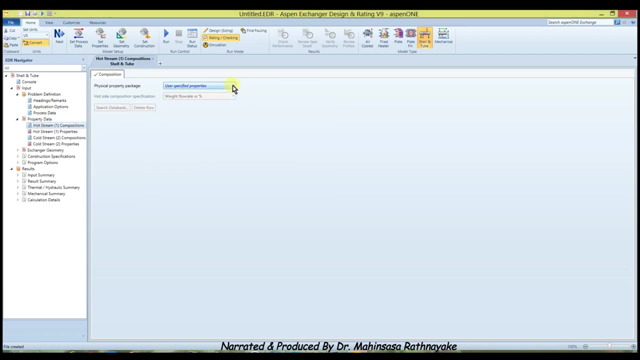 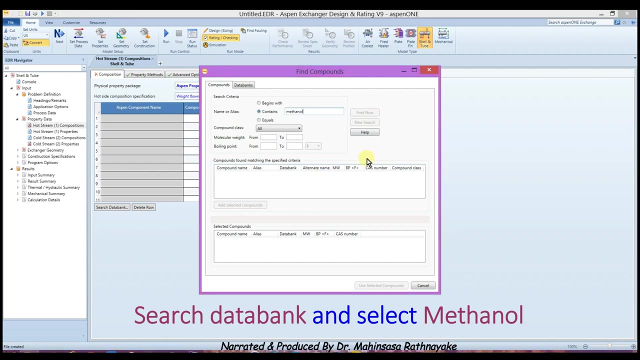 Then go and expand the property data option and select hot stream compositions. Select the physical property package as Aspen properties. Then click on search data bank and type our component as methanol. Select methanol and add selected components and select it into our list. 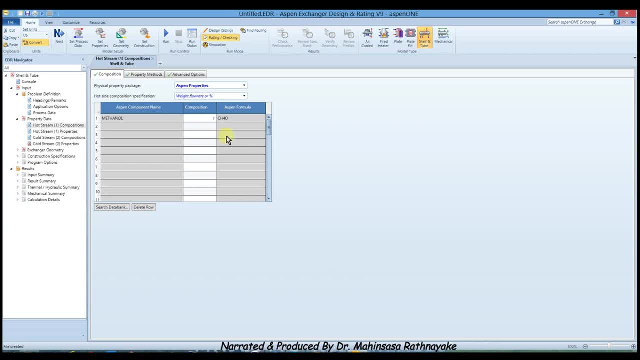 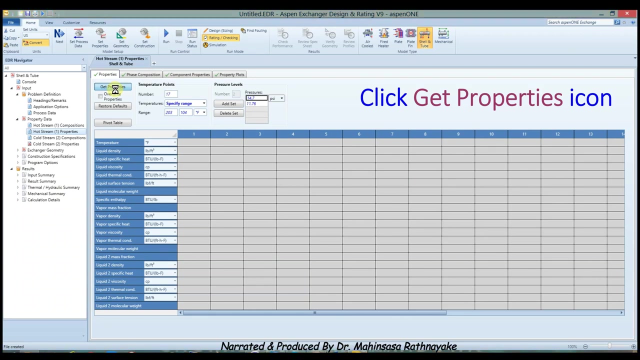 Enter the composition of methanol as 1.. Then click on property methods and change the property method to be NRTL. Then go to hot stream properties tab and click on get properties icon. Select all required properties as Aspen properties. The properties are displayed in the feature menu. 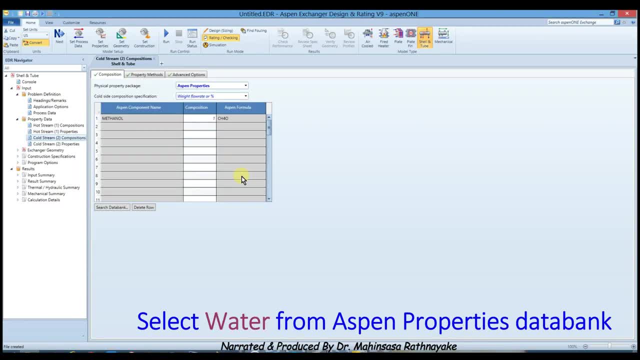 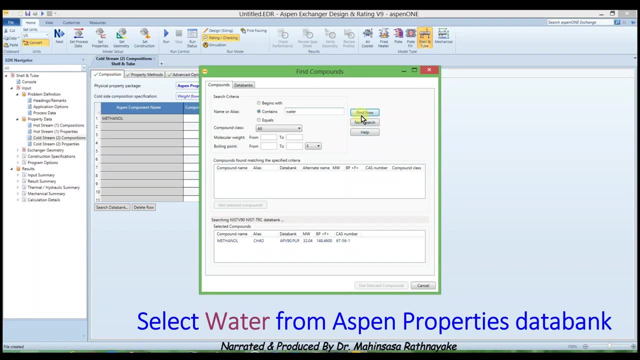 Then go to cold stream compositions tab and again select the physical property package as Aspen properties. Then click on search data banks and type water and select it into our list. Then enter the composition of methanol as 0.ㅑ. Select water as 0.ㅑ. 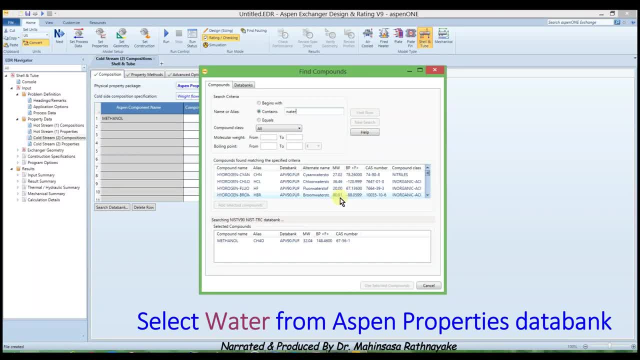 Then enter the water as 0.nm. Then enter the composition of methanol as 0.nm, Then enter the water as 0.nm. Then enter the hot stream water as 0.nm, Then enter the water as 0.nm. 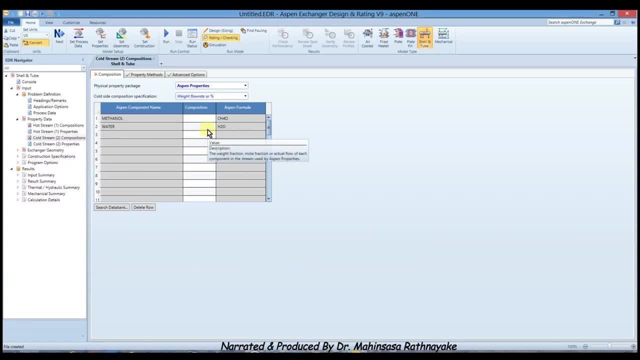 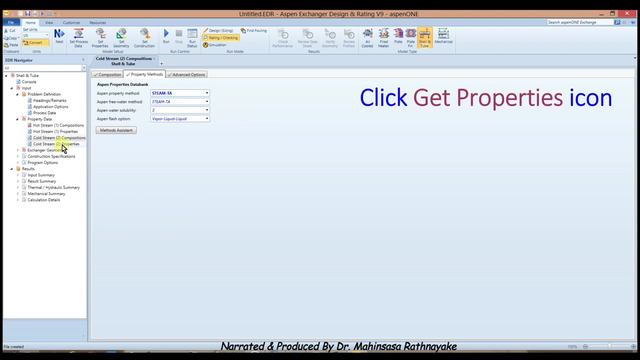 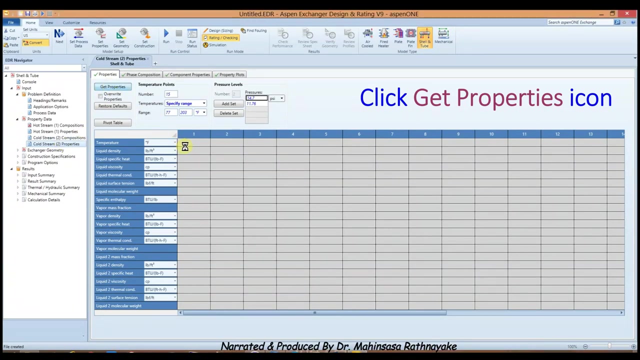 Composition of Water as 1 for the Coal side. Then go to Property Methods tab and select Steam TA as the Property Method. Then go to Coal Stream Properties tab and click on Get Properties. when all the acquired properties for water will be displayed, We can observe that again, Hot Stream Composition is displayed as Red. 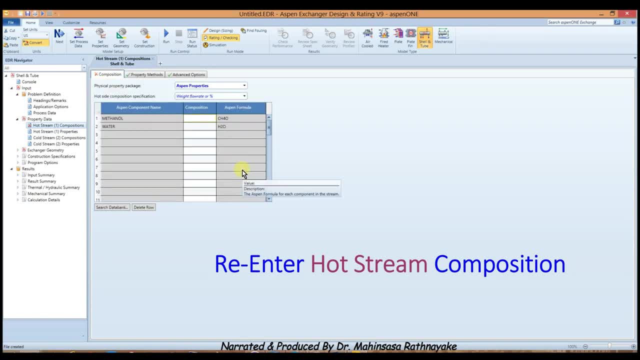 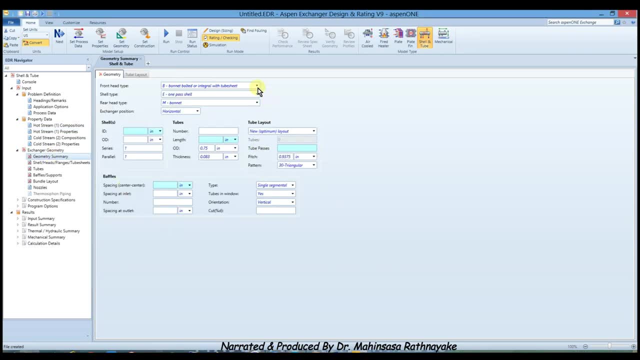 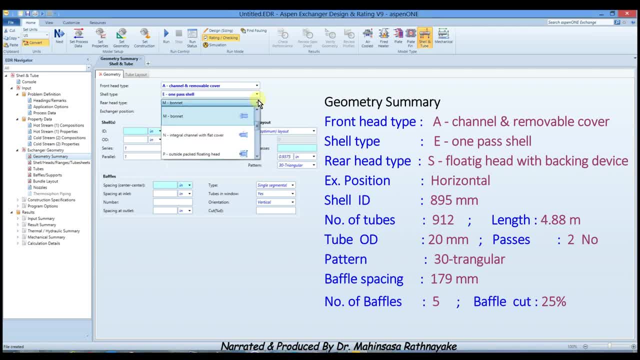 Rear Head Type as Floating Head with Back In Device. Let's keep Exchange Position as Horizontal and enter the Shell Internal Diameter as 895 mm, So the Outer Diameter will be displayed as 919 mm automatically. Then enter the Number of Tubes as 919 mm. 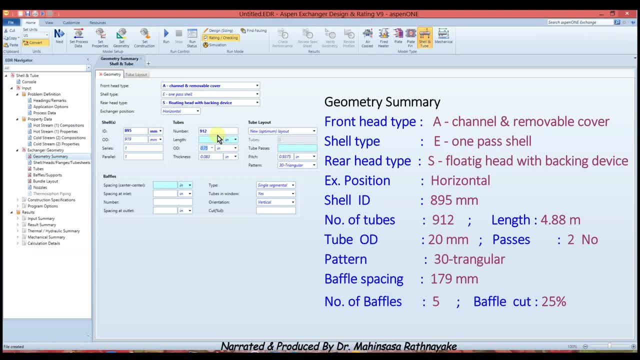 Then enter the Number of Tubes as 919 mm. Now enter the Number of Tube as 312 and length of one Tube as 4.88 m. Enter the Outer Diameter of a Tube as 20 mm and enter the Thickness as 2 mm. 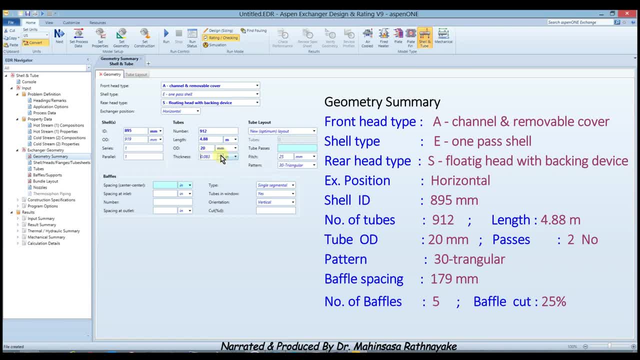 Next income字 i-iamp Automation, которая Playing i-i-i mean the Twenty Millimeter, is a 2 mm. Then enter efficiency and wp trong of the Tube. Enter: the tube passes as 2.. We can observe that the tube pitch is automatically selected as 25. 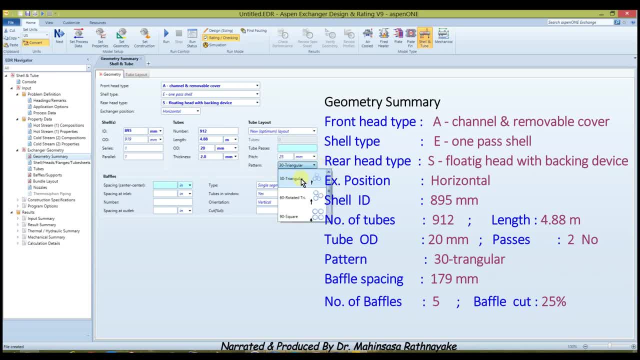 millimeters, so we don't need to change that. and also let's keep the tube pattern as 30 degree triangular. Enter the baffle spacing as 179 millimeters and number of baffles as 5.. The baffle type should be single segmental and our tube should be in the baffle window. 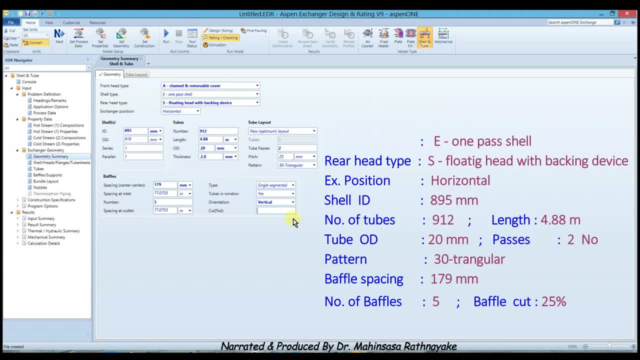 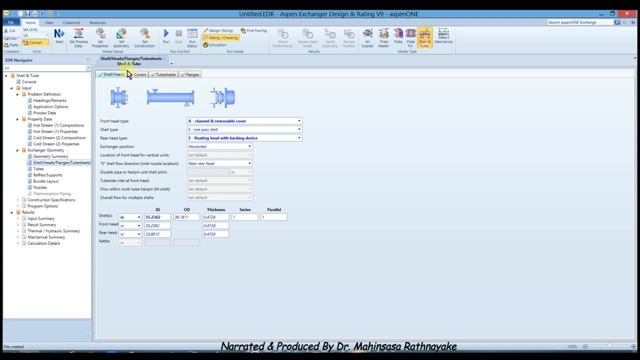 Enter the orientation as vertical and also enter the baffle cut percentage as 25.. Then go to our shell heads, flanges, tubes tab. We can observe that all the selected data have been filled in in this sheet also. Then go to tubes tab and change the tube material as copper, nickel. 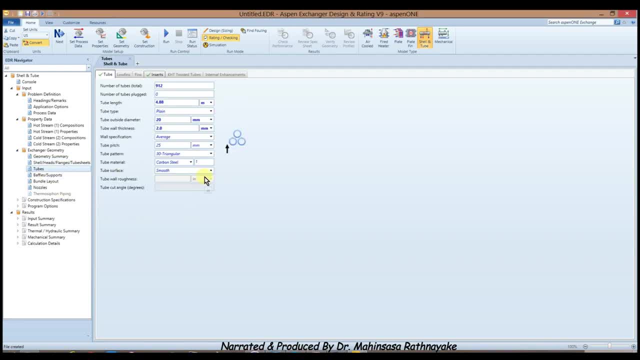 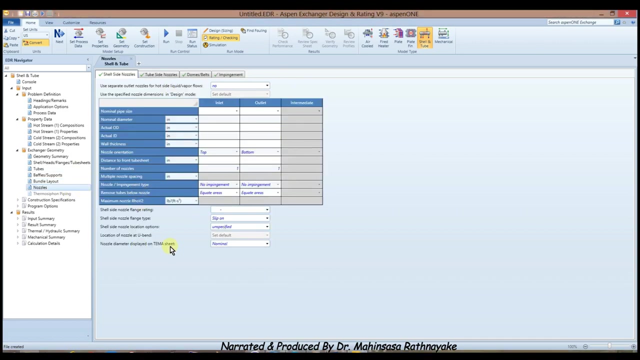 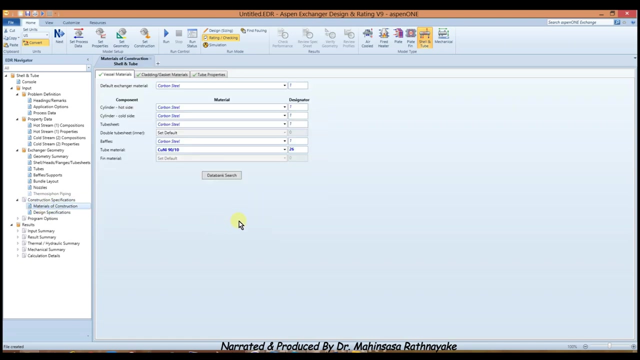 alloy of 10% nickel For the tube surface. select use specified roughness for our selected material. We can observe all the data have been filled in other sheets. Then expand the construction specifications tab and select on materials of construction. We know that the designator for copper nickel alloy of 10% nickel is 26.. So type designator. 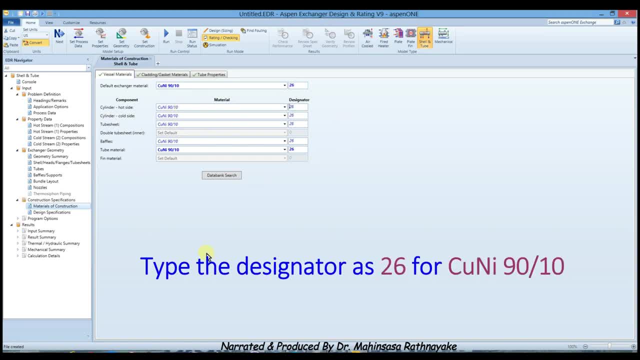 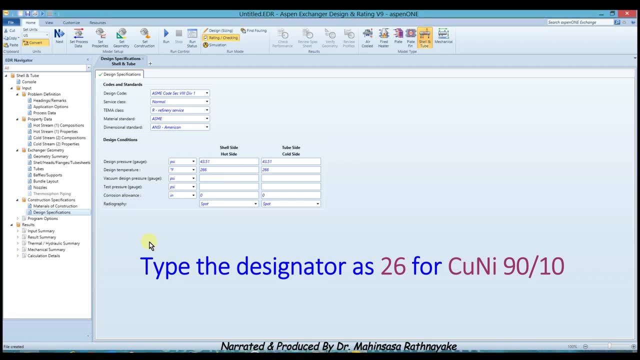 at default exchanger material as 26.. So we can observe that all the exchanger material change into our required copper nickel alloy. Then click on design specifications. We can observe that the design code used for the design of our heat exchanger is ASME code, section 8.. Select the service class as normal, TEMA class as chemical service. 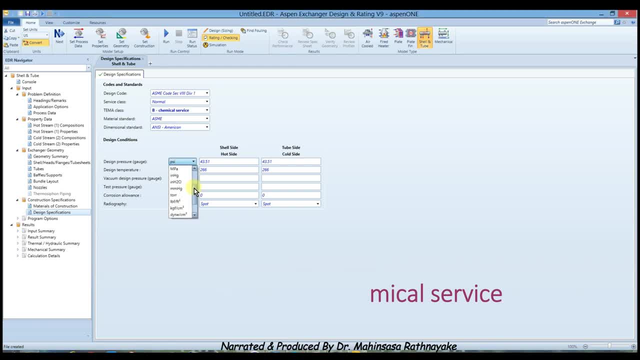 We can observe that design pressure and design temperature have been already selected by the program based on ASME code, section 8.. Keep all other tabs as default. We have a specified all the geometry data for our heat exchanger design. Let's click on next and. 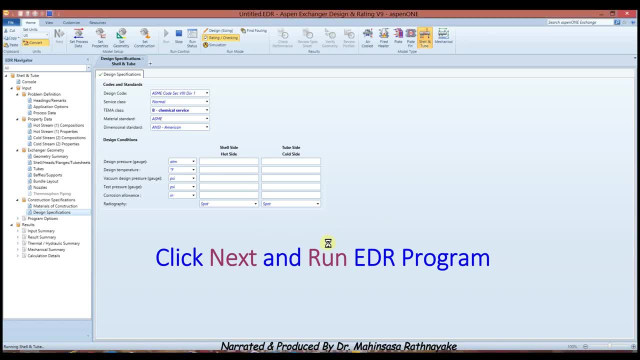 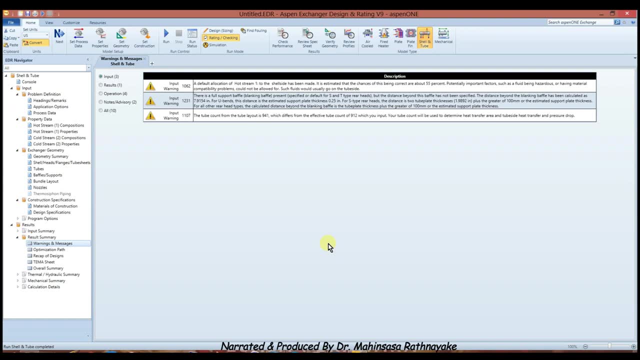 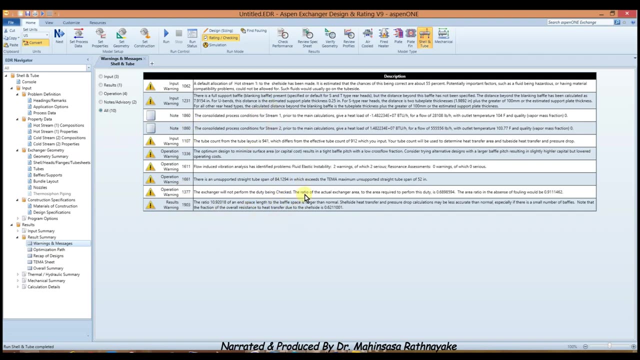 run the Aspen EDR program, We can observe that some suggested warnings have been created from the program. Reading these warnings will be helpful for further amendments of our design to obtain the most suitable design. Note that the program suggested that the number of buffers we have used is not enough and 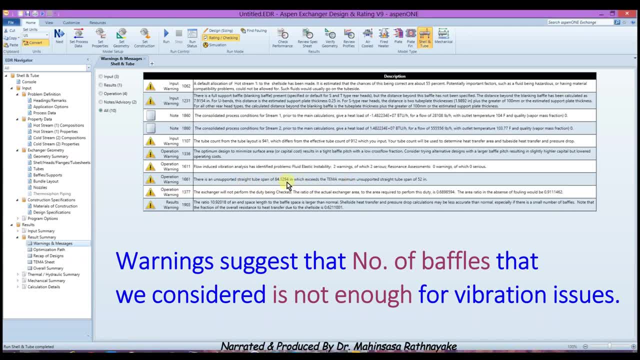 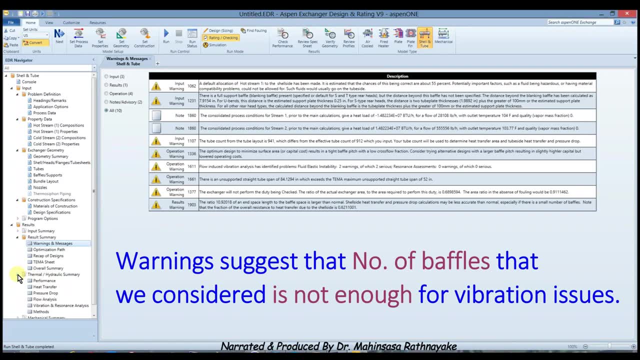 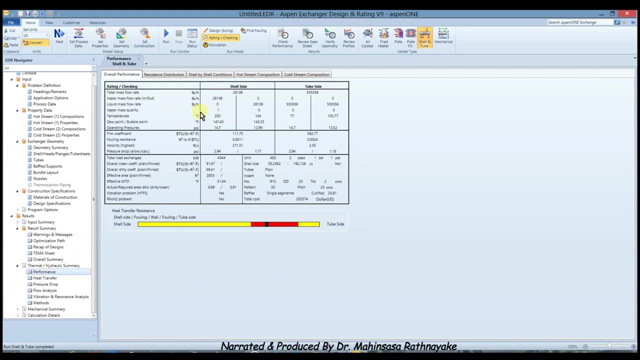 it will create some vibration problem with our heat exchanger. We can observe the results for the overall coefficients in the thermal hydraulic summary performance tab. According to the shown results, The results are closer to our manual calculations. However, the program suggested that there is a vibration problem and also heat exchanger. 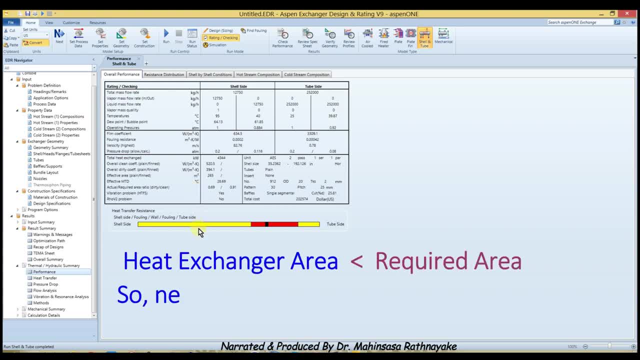 required area is less than the actual required area. Therefore, to obtain a proper design, we may need to amend some geometry parameters of this heat exchanger. In that case, as chemical engineers, we need to get the help from mechanical engineers, who actually decide the geometry. 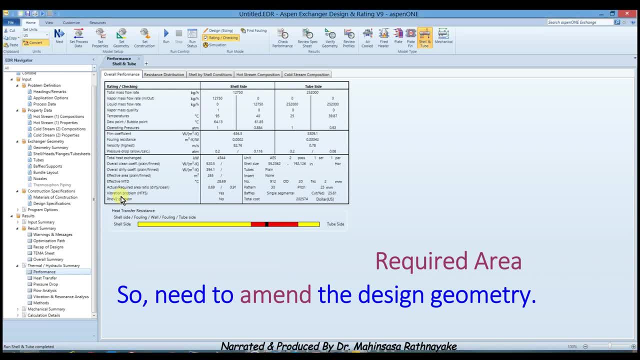 for the heat exchanger. We can also observe that in manual calculations we didn't consider any coefficient specifically for vapor phase and liquid phase. However, in the Aspen program it actually calculates based on the different phases. This may be the reason for slight deviations of manual. 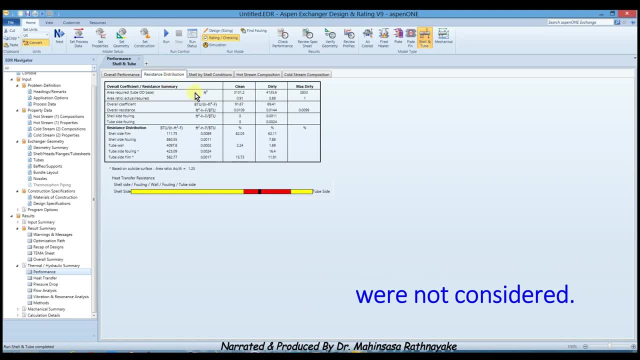 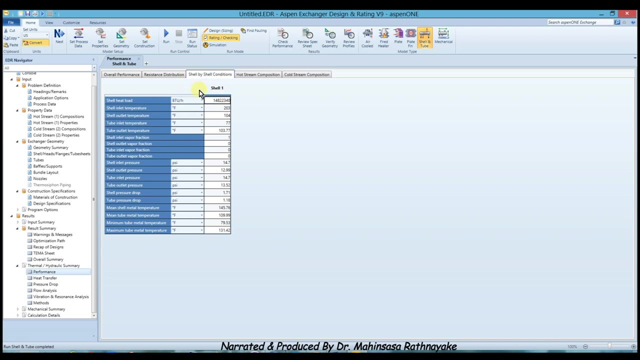 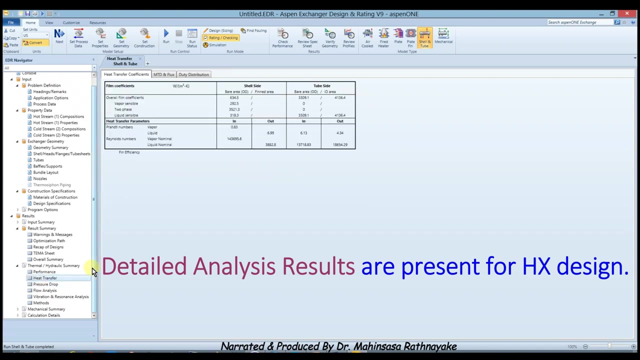 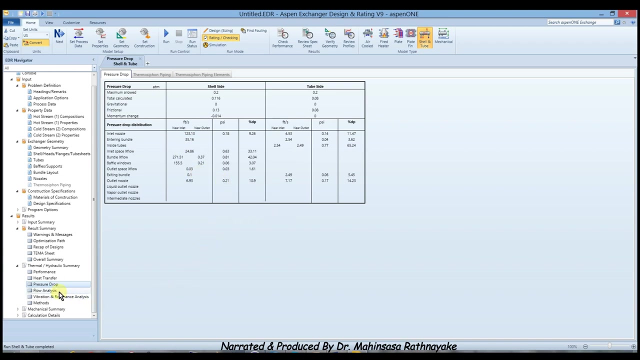 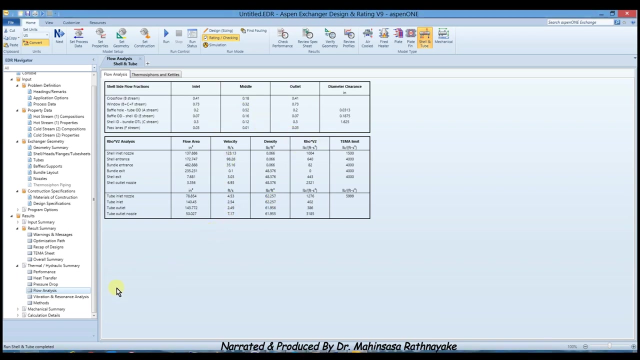 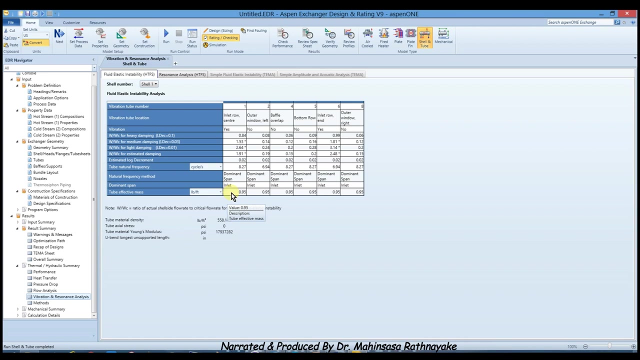 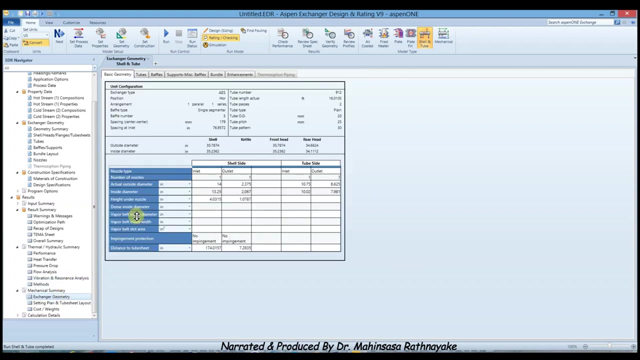 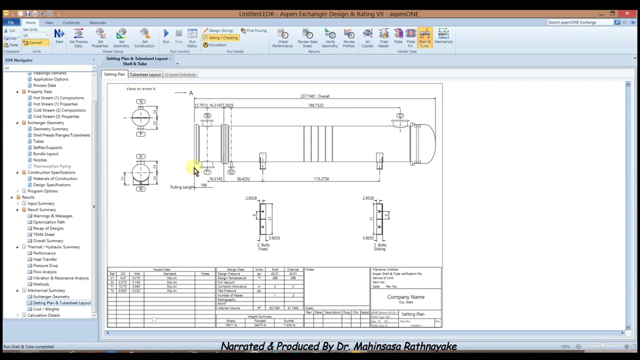 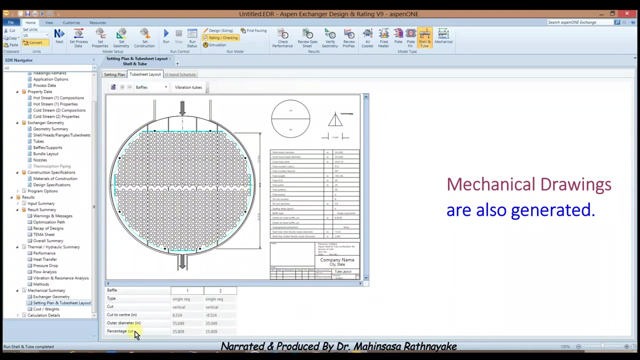 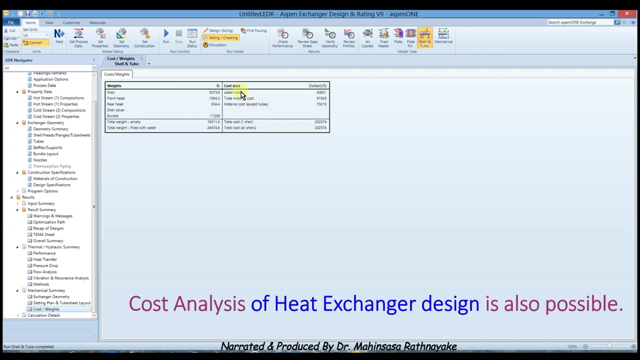 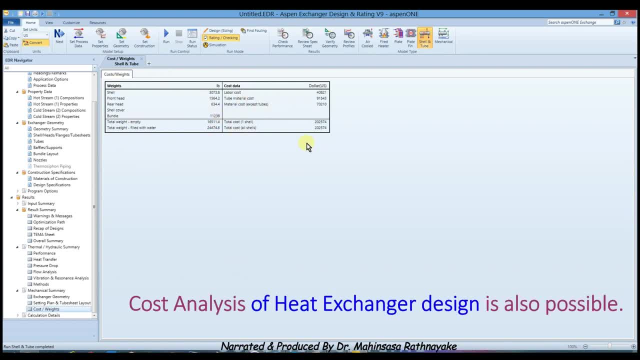 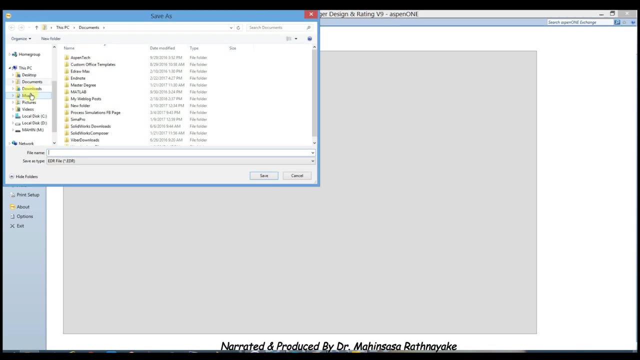 If we know the pricing of our materials and capital cost, we can plug in those data into this program and find out the actual cost. That step can be used in the future design simulations. Now save this generated EDR file in a desired location and go back to Aspen simulation, which we previously created using the shortcut method. 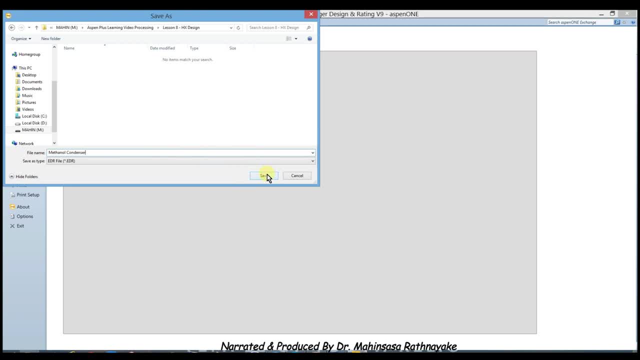 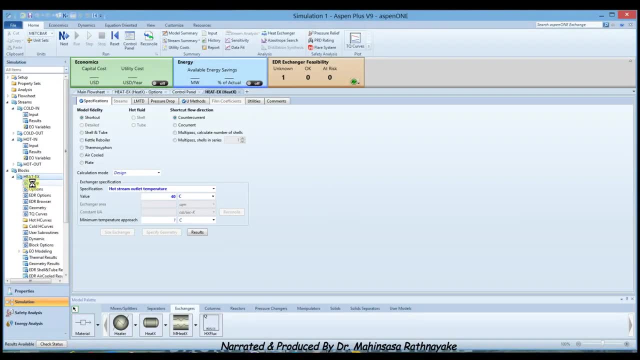 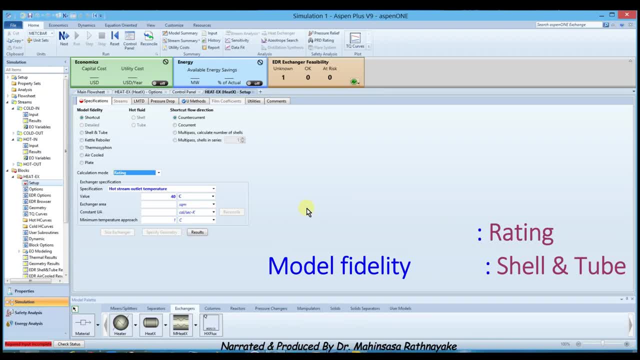 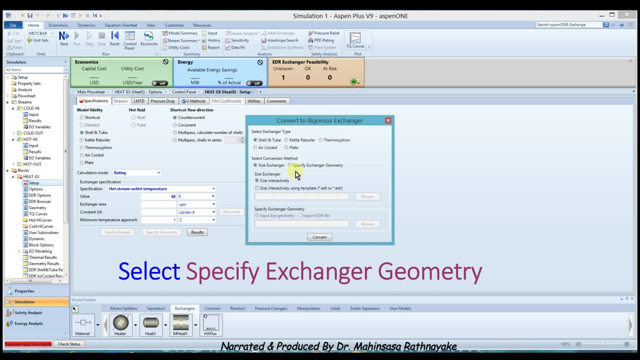 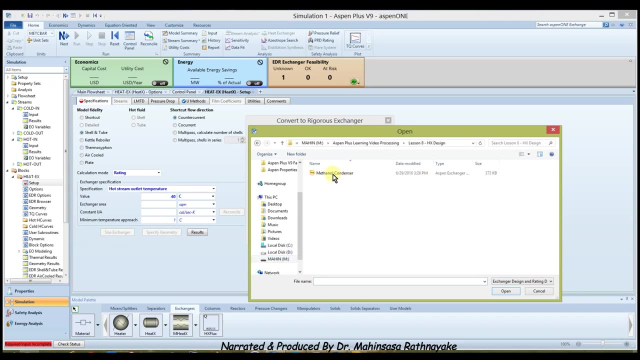 Change the Calculation mode into Rating and change the model fidelity. Then convert to rigorous. exchange window will be opened. Select the Conversion method as specify exchange geometry freedom. Click on To Input EDR file And browse the EDR file which we saved inside our desired location. 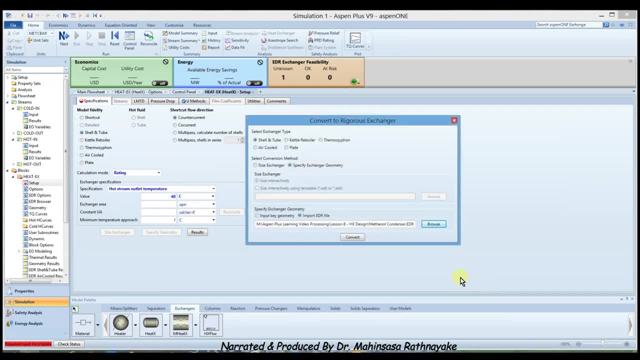 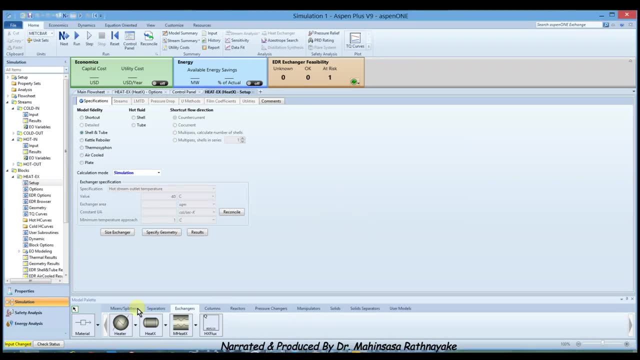 Then click on Convert. Aspen Plus asks us to change the input, so click OK. Now our EDR design has been inserted into our Aspen simulation. Click Next and run the simulation. We can observe that one warning is present. It says a possible vibration problem has been identified. 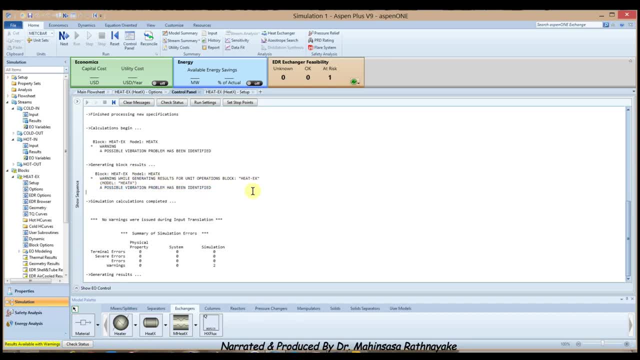 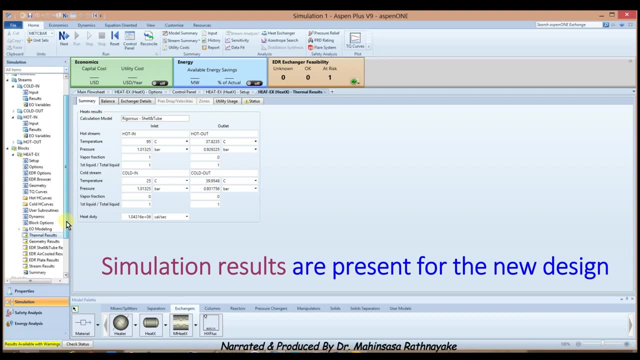 As we previously observed in EDR program, the reason for this vibration problem should be the lesser number of baffles we used. Now we can observe that the overall results have been changed in Aspen simulation, Since our heat exchanger area has been changed. 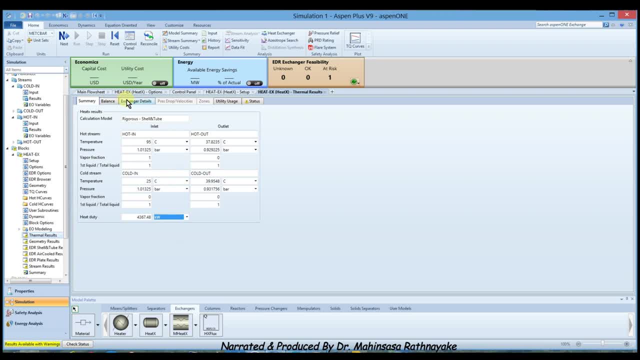 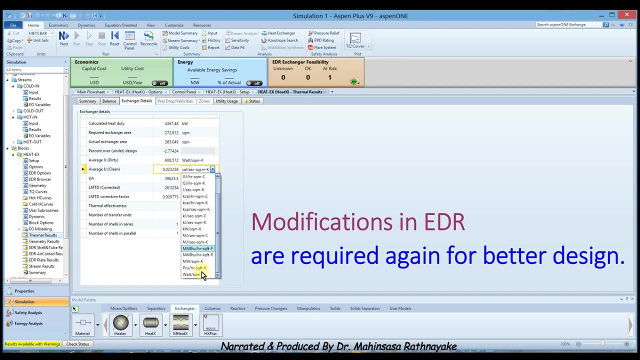 parameters have been changed accordingly. However, we can observe that these simulation results are closer to our manual calculations. In order to obtain the best suitable design for our heat exchanger, we need to change geometry parameters again in the EDR program and find out the most suitable design. This step will be performed by mechanical engineers.